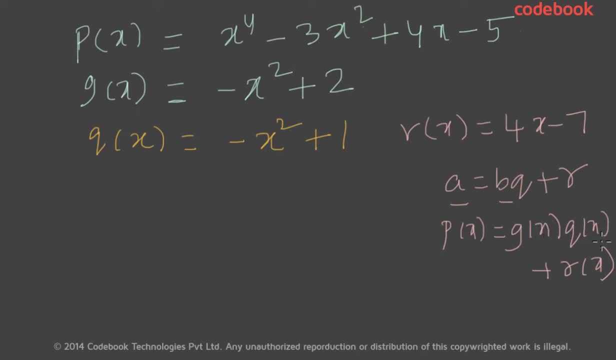 that. So let us start with the right hand side. So right hand side is g of x times q of x. So g of x is minus x square plus 2.. And multiply that with q of x, which is minus x square plus 1, plus r of x, which is 4x minus 7,. 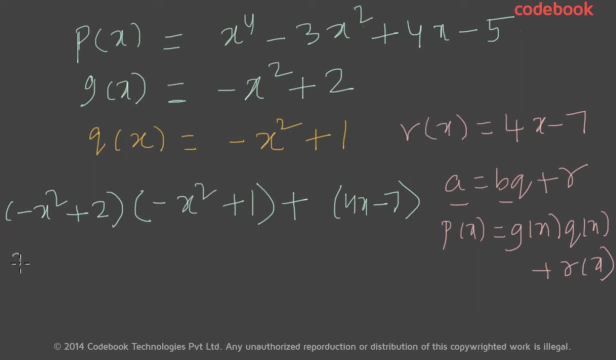 right, So multiply this. So minus x square times minus x square is x power. 4.. Minus x square times 1 is minus x square. plus 2 times minus x square is minus 2x square. plus 2 times 1 is plus 2, and. 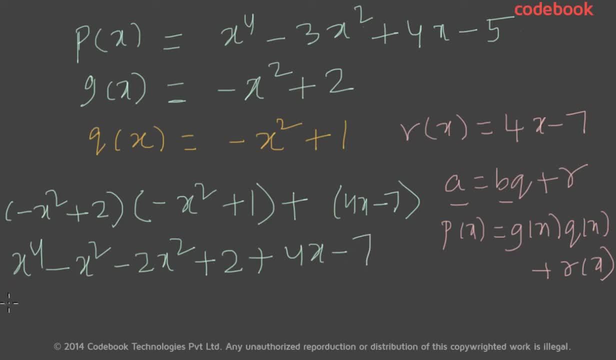 plus 4x minus 7.. So if you simplify this, x power 4, you have two terms of x, square. So let us add them up: Minus 3x square plus 4x, right? So the next term which has x is 4x. And then you have the two constants which are 2 minus. 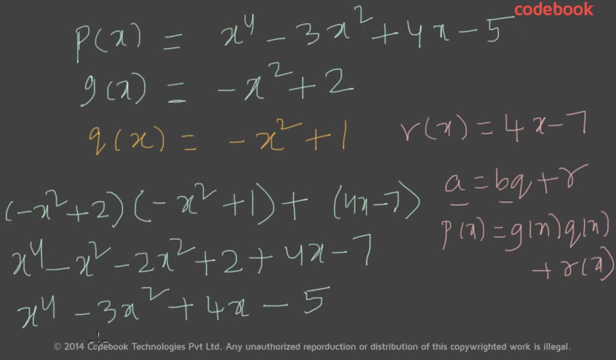 7, which becomes 2 minus 7 is minus 5.. So, if you observe this closely, x power 4 minus 3x square plus 4x minus 5 is nothing but your p of x, right As you see here. So this equation is actually: 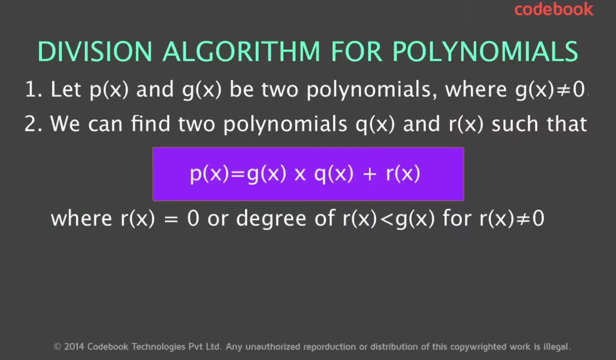 true for polynomials as well. So now let us try to formalize the previous finding. So the division algorithm for polynomials, So this is Euclid's division algorithm, right? So the step one is: let p of x and g of x be two polynomials where g of x is not equal to 0, right, Because anything. 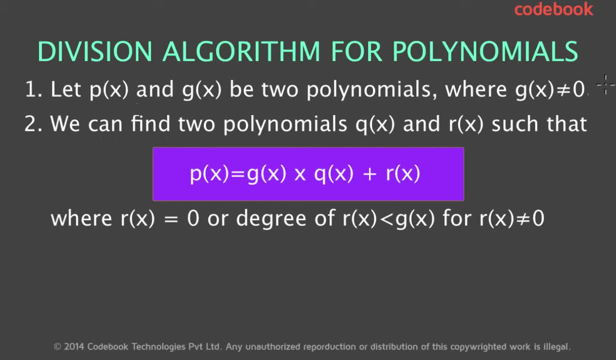 divided by 0 is undefined, So g of x should not be equal to 0.. So then we can find two polynomials, q of x and r of x, Such that p of x is equal to g of x times q of x plus r of x. We have just verified that, And if 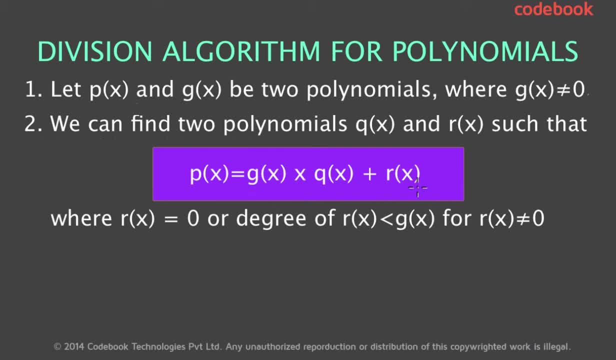 you recall, q of x is a quotient and r of x is the remainder. So we have also learned in the previous lesson that the degree of the remainder should always be less than the degree of the divisor. In this case, the divisor is g of x. So here we are saying exactly the same thing Either.